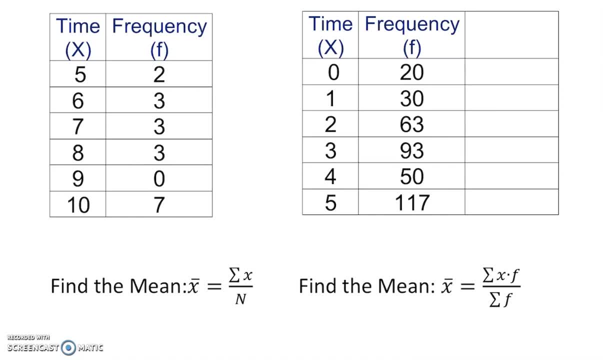 actually, here you go how i'm gonna pull out the data. so this one is basically five shows of twice. okay, easily I can show five, five, five and six. look at that. six- how many times shows up? three times six, six, six and seven. also three times one, two, three, eight, also three times eight, eight, eight. 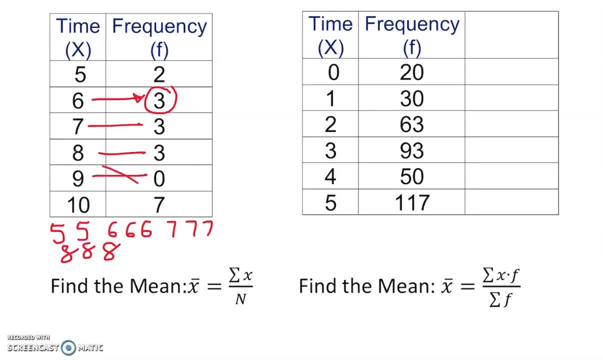 nine, none, okay, none, ten, seven, one, two, three, four, five, six, seven. you got the point. I can just extract all of them. okay, I can just extract all of them. now, if I do extract all of them, my sum of X wouldn't be 143 if you add all of them. 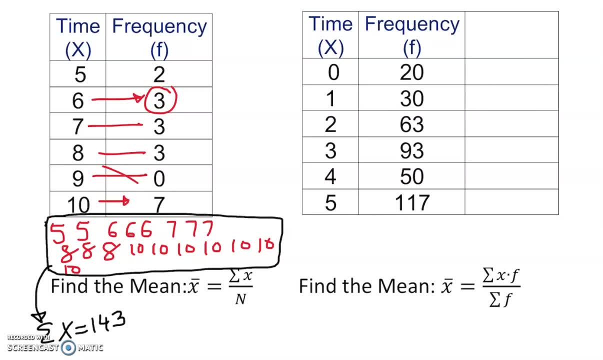 one hundred 143. so guess what? I do have my Sum of X. I just add that traditional law, which is 143 over Total number. So how many number? let's actually work it out here. How many numbers right? 1, 2, 3, 4, 5, 6, 7, 8, 9, 10, 11, 12, 13, 14, 15, 16, 17, 18. 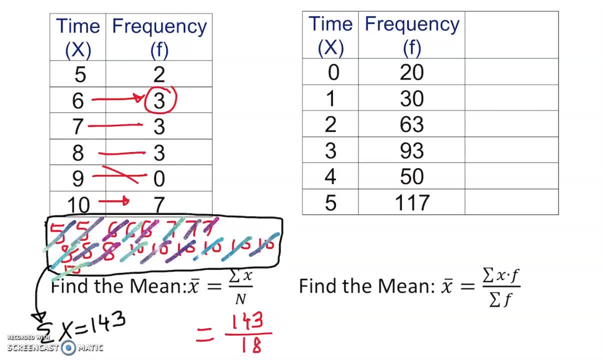 Bingo. we have 18 number and If I divide it with half of any calculator or do long division, right, Basically we should get seven point. We should get seven point. Let's do this one for the seven point. nine four Nearest hundred. you got the point right. 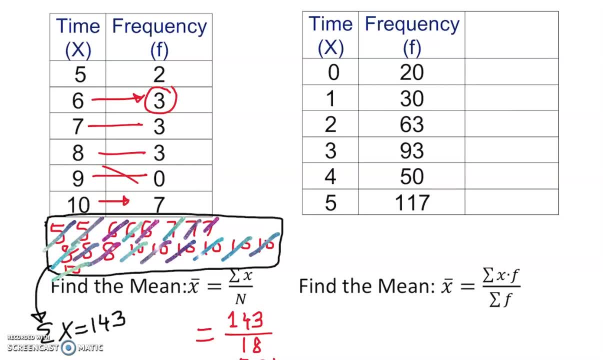 Now we look into the other one. Okay, so if you look into the other one, look, Zero shows up. how many time look so many zero. right, One, two, three, four. you got the point? Okay, You got the point and it goes: five, like that is going like that and like that, and of course, five, five. 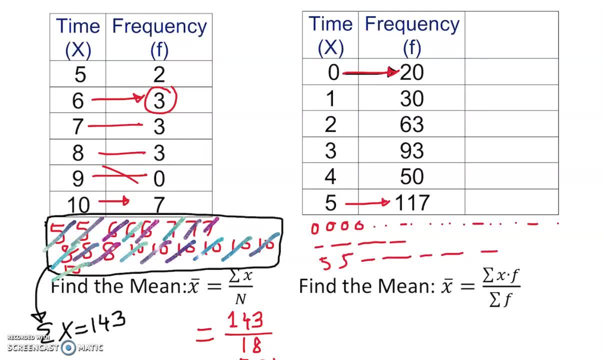 I can even fit five here, hundred and seven in time. We cannot do this. It's not going to work. not Gonna work. Okay, it's not gonna work. So we have to come up with a little bit smarter way of doing this. We've got quicker way of doing again, guys, I'll make sure that you understand that. this is like when we learn addition, right? 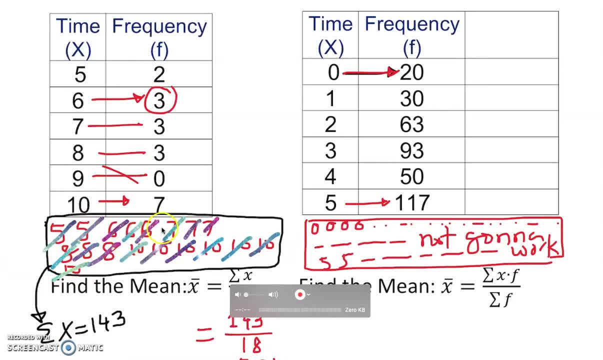 You just do slowly, you just add it right. when you do multiplication, you do faster. Well, that is the reason we're gonna. that is what we're gonna do. So we're gonna multiply this, actually. okay, I'm gonna multiply this Zero times 20, so X times the frequency, X times the frequency again, that is here, this one we are working on here, okay. 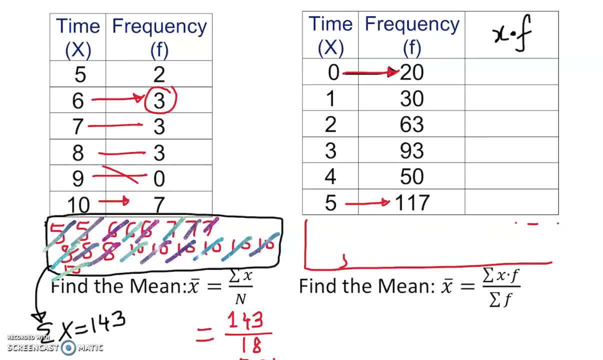 So I this is not gonna work, So definitely I'm gonna erase that. okay. but to come up with a clever idea, clever way of Finding the mean from frequency change table: Okay, so if I just multiply them right is gonna be 0, 30. 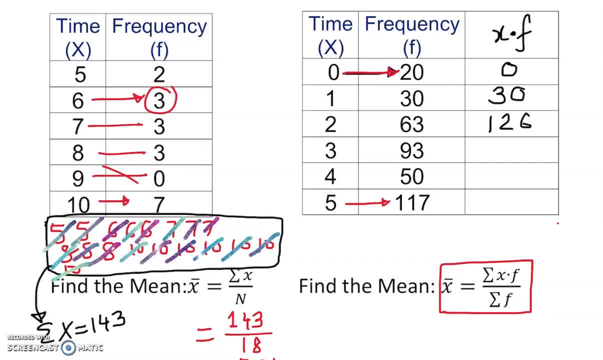 Of course, 126, 3 times 93, 279, 4 times 5 is 20, 200 and 5 times hundred, 500. and of course, 517 is 585.. So 5: 85. look so this symbol. I want to make sure you understand that this symbol summation means you add all of them. 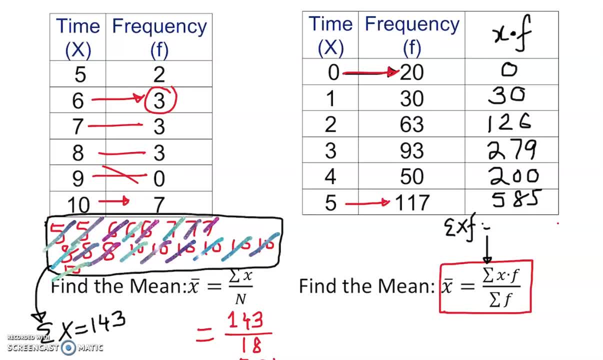 So this is going to be sum of X times the frequency equal to: Again, you take a little half of any calculator, right, It should give you 1220, 1220. check that out with you calculator or do it manually. Okay, so guess what guys? we already have this here and 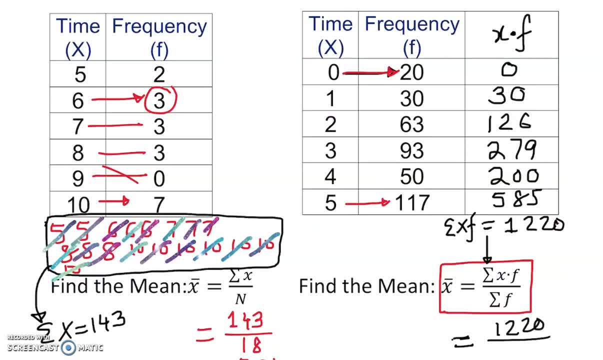 so, So 1220. Oh, Here we go. That should be you N, while instead of n. I want to make sure that we understand, so you see it. so, on this end, That's basically same thing And is total number. so I'll. how do you find total number? remember this X. 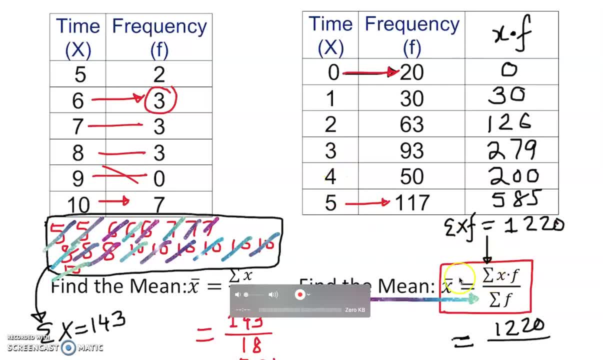 This X is not going to give you total number. Okay, This X is not going to give you total number. Or, if you add, this X is not going to give you. adding this sum of x is not going to give you that you have to multiply. this is your sum of x. 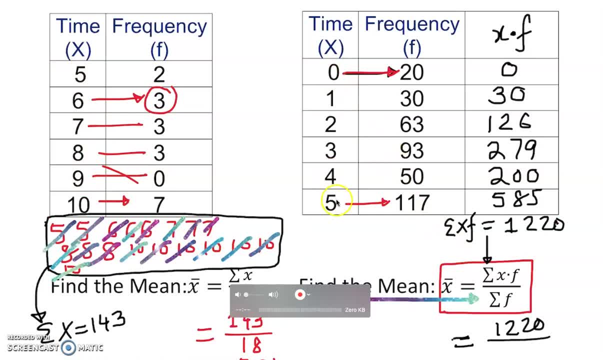 not from this one. so same thing we do. you don't add this, you multiply, then add. this is basically equivalent to the sum of x. okay, sum of x times frequency: the same as same of sum of x. now, this sum of frequency is basically: give you the total f. okay, it's give you n. so if i look here, sum of f.